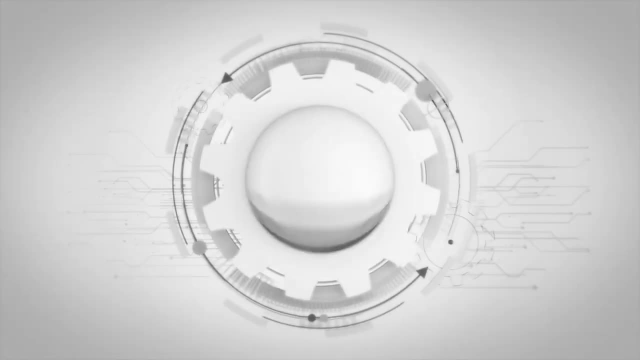 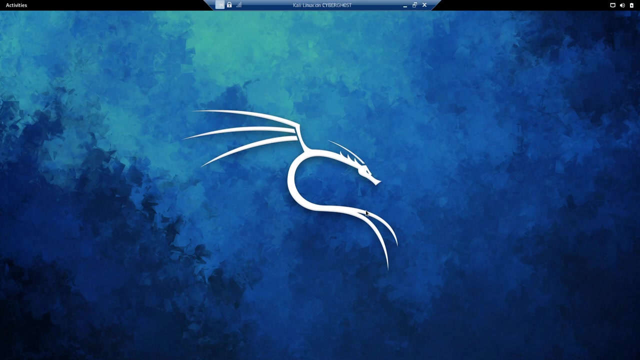 hey everyone. i hope you all are doing good and having a wonderful day. in this video, we are going to learn everything related to race condition vulnerabilities like: what is this condition vulnerabilities? where do we look for these kind of vulnerabilities? what is the root cause behind these vulnerabilities? and a lot more right. but, as always, before going to this video, if you haven't, 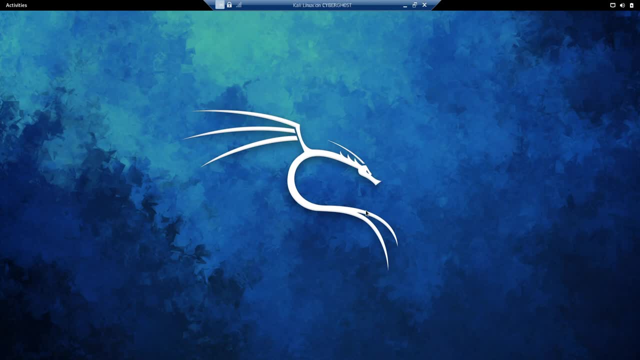 checked out my previous video, in which i've shown you that how we can find hidden informations in a javascript file using a tool known as mantra. then go ahead and check it out. the link is given in the description as well, as you can see it on the right side of the screen. and now, with that, 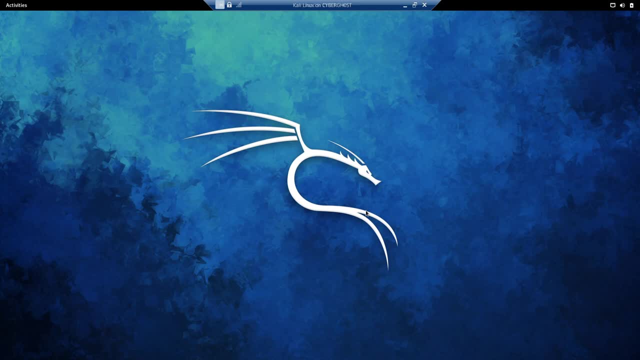 being said, let's get started. so first thing, first let us try to understand what is race condition, vulnerability? basically, in simple terms, we can say that suppose there is an application right where you are allowed to, you know, create two or three accounts. or let's take another example for 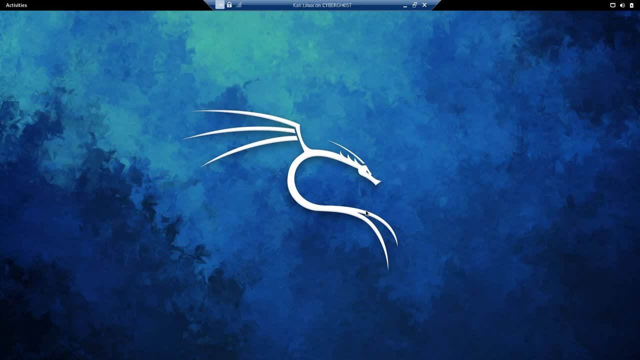 example, let's say there is an e-commerce application where we have a functionality to use coupon codes- right, we all know that coupon codes generally expire after using it for one time, right, or maybe two or three times, depending on the coupon right. but what will happen if the 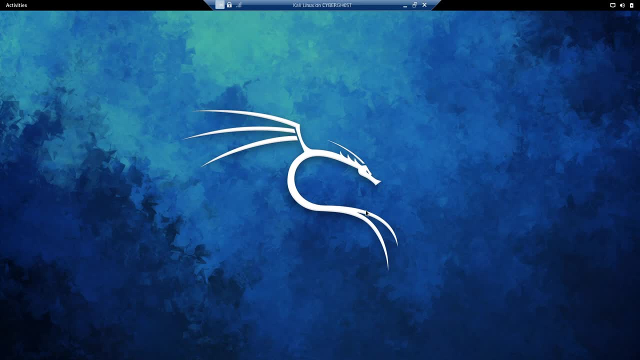 attacker is able to use that coupon multiple times. but let's say the limit is one, right, for example, the coupon code you can only use once. right now, what will happen if the attacker is able to use that same open code twice, right? in that case, he will be able to, you know, break the logic of the application and 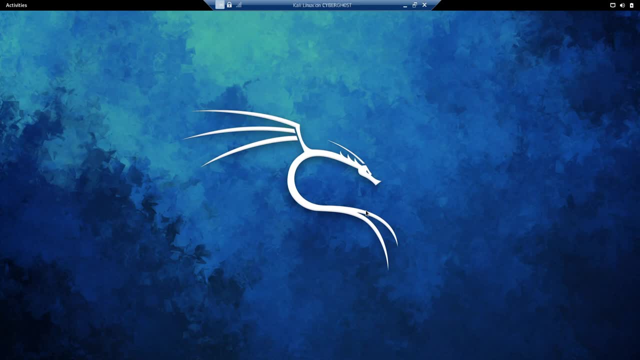 the root cause behind this vulnerability is race condition vulnerability. we'll go deep into this term- race condition- but first let us try to understand this with an example. so, for instance, i have created a lab. let me show you so. let me just open my browser here and let me just go to. 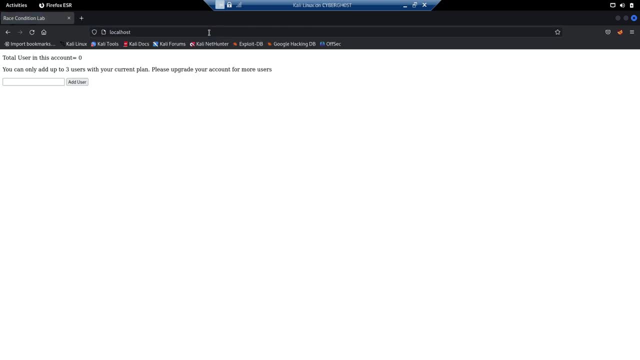 localhost, and this is the application that we are going to test for this condition: mobility. let me just minimize this and now see this functionality over here. we have: total users in this account is currently zero and it's saying that you can only add up to three users with your current plan, right? 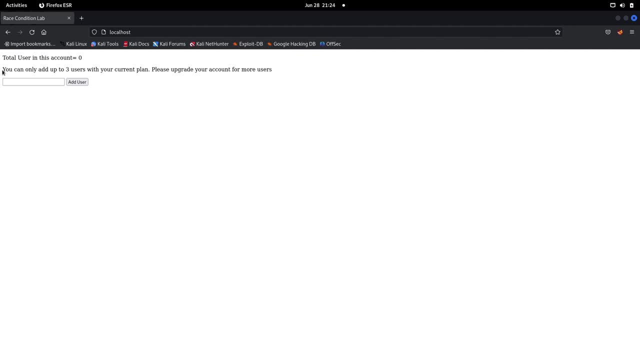 so let's say: this is a application in which you are allowed to only add three users, right? if you want to add more users, you have to upgrade your account or you have to buy the subscription plan, right? something like that. so the three users, only three users are. 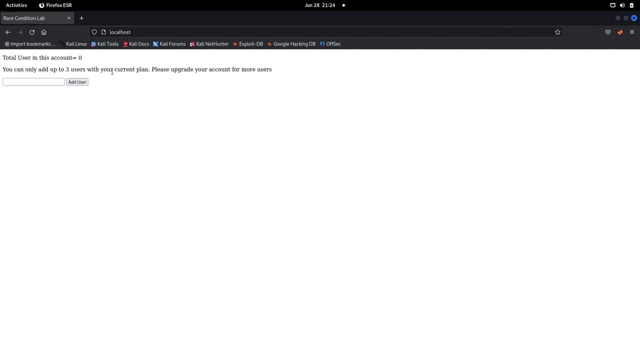 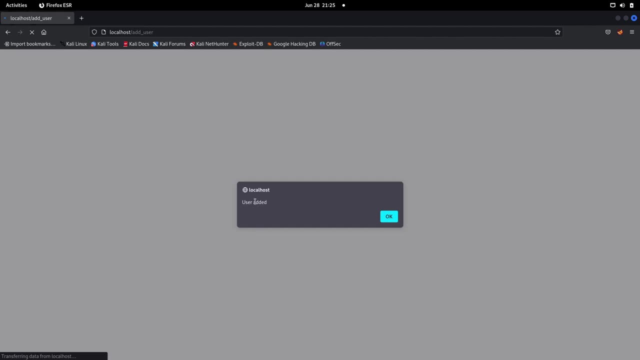 allowed right, which means that the max users, the max amount of users that we can create, is three. let's try to create the users. for example, let's say the first user is myself. as you can see, it is saying that the user has been added right. let's try to add another user. let's say: be practical. 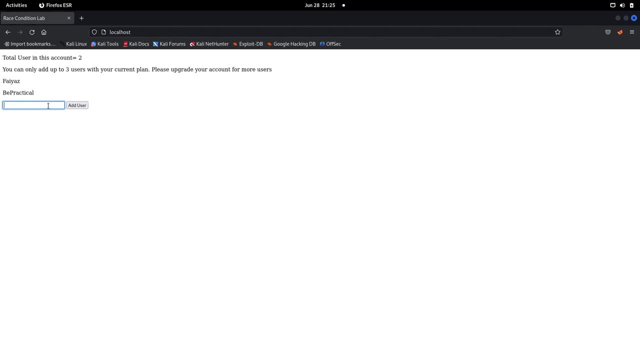 let's add this and let's try to add another user. let's say, uh, testing right. as you can see, we have added three users. now let's try to add more users. for example, testing two right. let's click on add users and, as you can see, right now we get a message saying unauthorized right, which means 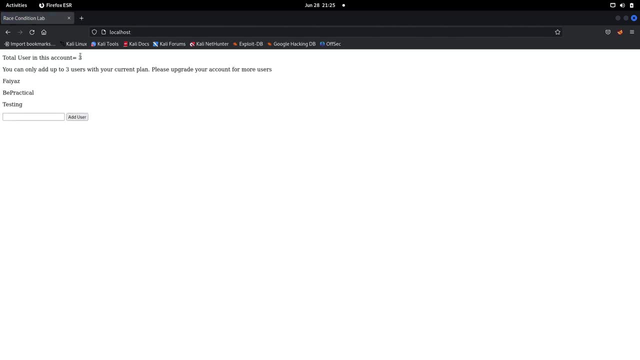 that we are not allowed to add users more than three, right? if we want to add it, then we need to add more users, right? this is what this application is saying now, how can we bypass this particular functionality, right? sometimes if we send multiple requests to this endpoint, so it may be possible. 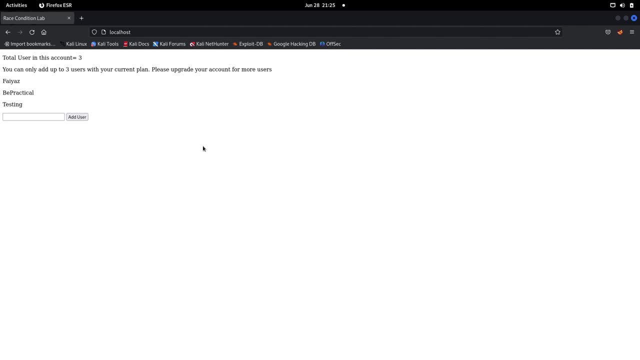 that we'll be able to add more than the limit has been set right, the more users rather than the limit that is set by the application. for example, here the limit is set to three right, which means that we could be able to add more users than three if we send concurrent requests, which means we send huge amount of requests at the same. 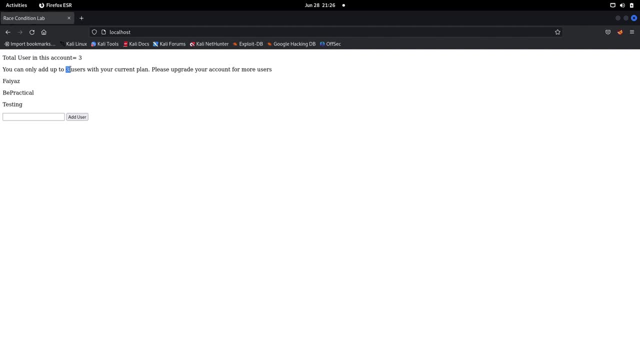 time. right. this is what race condition is all about. this is how you look for vulnerabilities: race condition, type of vulnerability, right? so always try to look for this condition in in that functionality, which have some limits, like the previous example, like the coupon codes, like this one, like here- we can only add up. 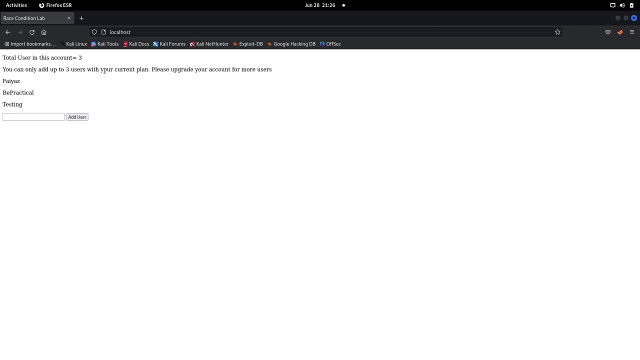 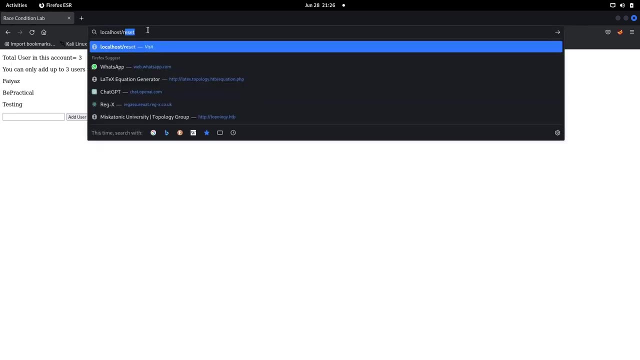 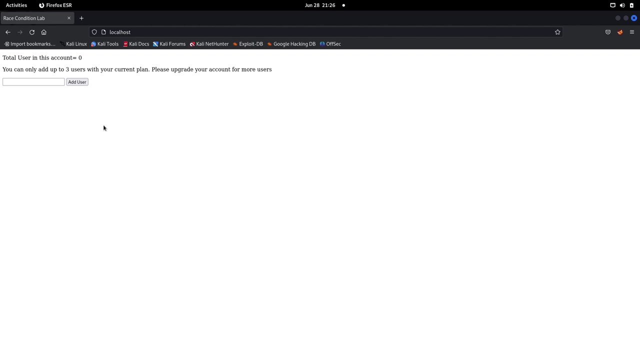 to three accounts, right. so these are the perfect scenario for testing race condition vulnerabilities. now let's try to add more users. see how we can find this condition in this particular application, so i'm just going to reset it to zero. we saw that we are only supposed to add three users, right? so if we were able to add 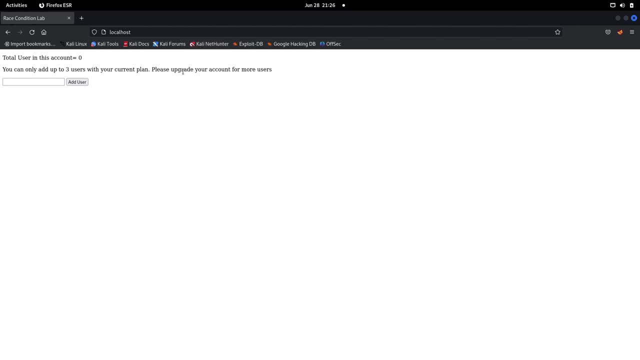 more than three users, which means that we are using the premium account functionality in our free account, right? so there is a business loss kind of vulnerability over here, right? so this is a logical, but let's try to understand that- how we can do this so that you can either use burp suit. 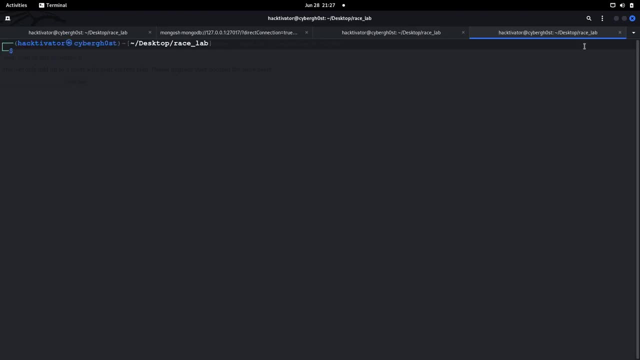 you can use a burp suits intruder or you can create your own custom tool written in python or any other language. in this example, i am going to write a python code that will help you to understand what we are going to do in this particular scenario. let me just go to my main directory. let's create a. 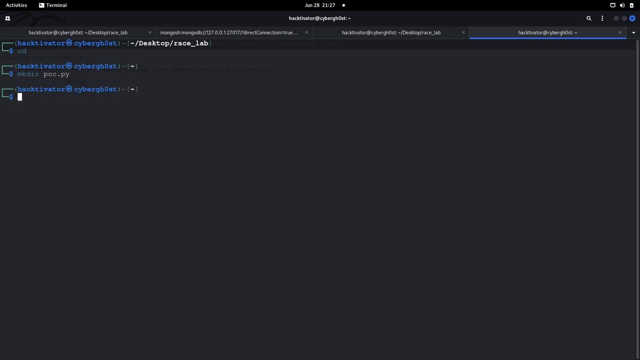 software. let's say pocpy. oh sorry, let me just create pocpy, right? okay, that's some mistake. let me just. let me just get rid of this dot py, and now let's create this. yeah, so now let's import some important libraries request and then we are going to import threading why we are going. 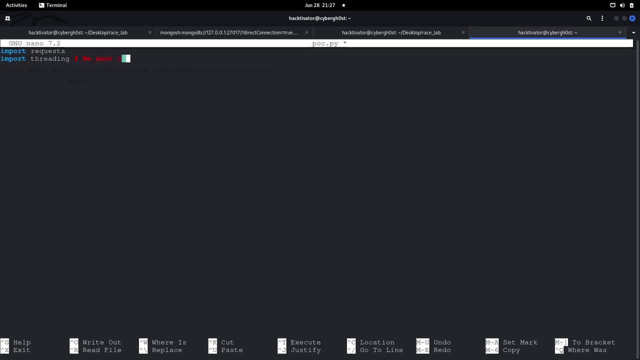 to import threading because we want to send- ah sorry, we want to send- multiple requests right to the server at the same time, right? this is why we are going to use threading in this particular scenario. let's specify the url. the url is that url which we are going to use to send the post request. we can either use burp. 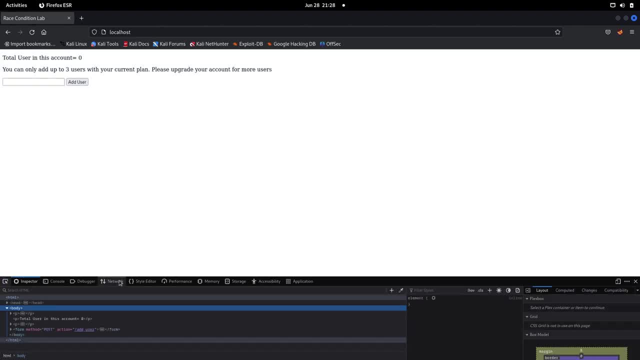 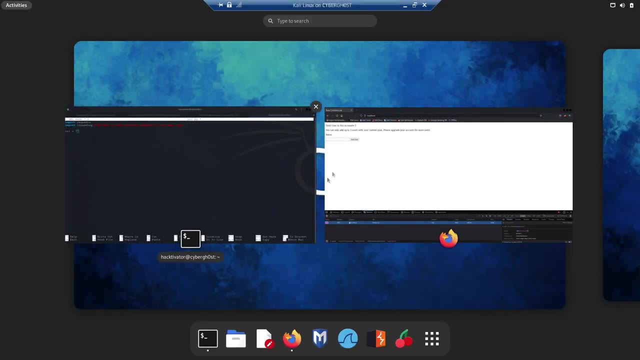 suit to find the url going in the post request, or we can just go to the network tab. let's add a user. let's click on add user and there we'll be able to see the user. okay, we are not able to see this. let's try to open burp suit. 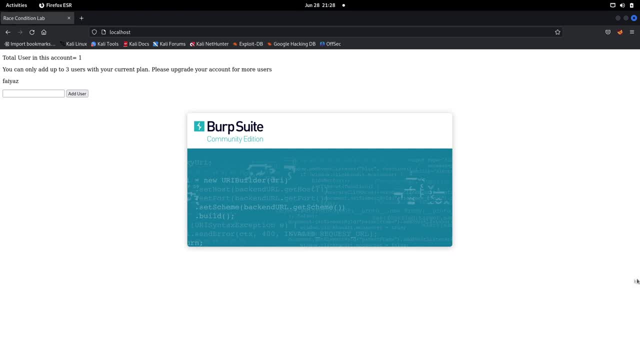 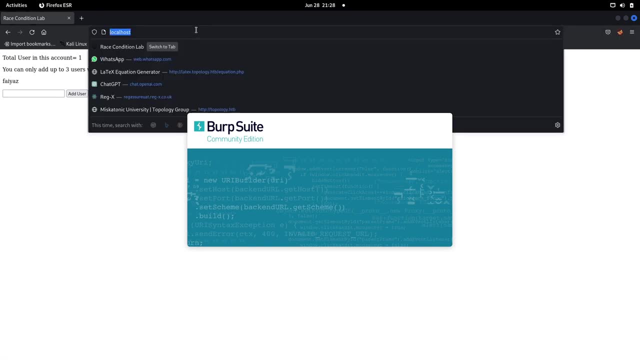 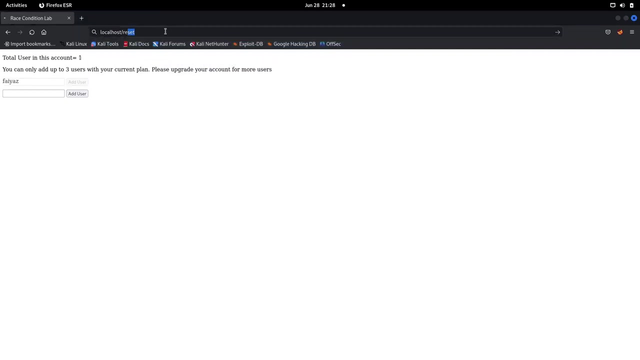 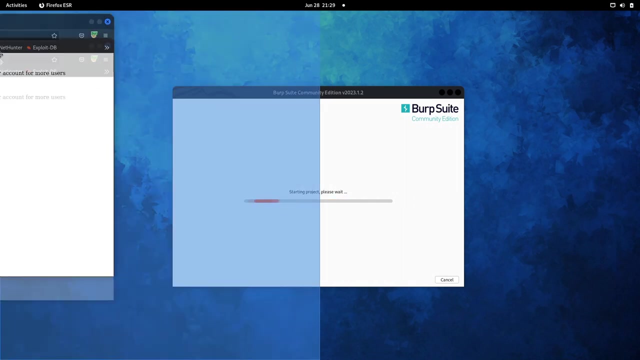 let's wait for a few seconds. let me just load burp suit really quick. meanwhile, i'm just going to reset it. start it like this: let's just reset it and just use the burp. here it is. here's our burp suit. let's turn on the interface. 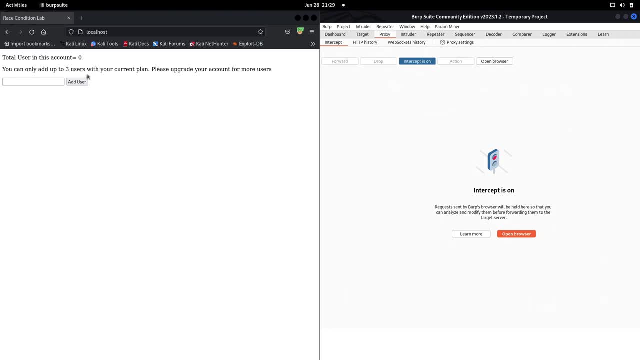 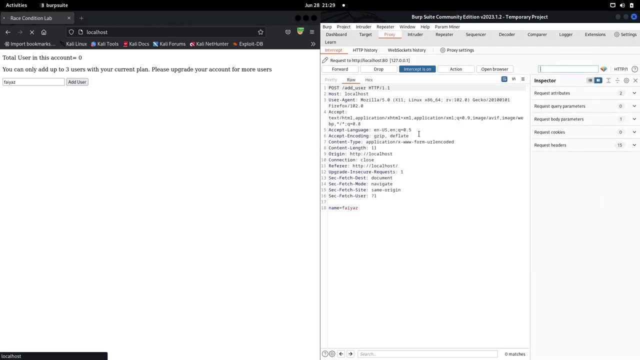 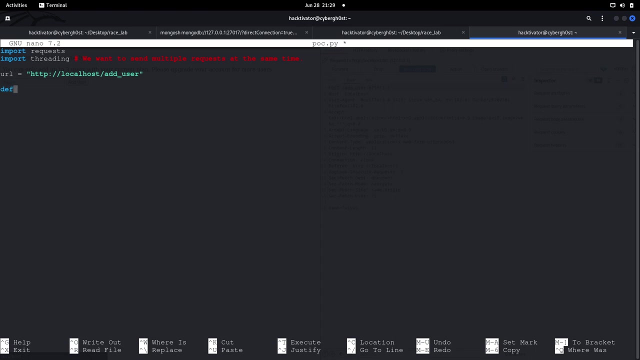 hit enter. we found here as a burp suit we actually can paste. we are going to know what is that mean and also use the elements to make pivot from the underlying. then we need to remember that because this citizen type field is already assumptive, this cabinet is: 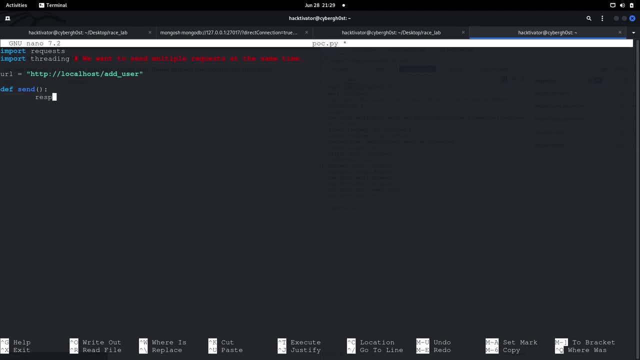 going to written with original plaisir, like if i need to run it again. I'm going to save the response to this response variable and with requestpost method, I'm going to send a post request using Python. So here we specify the URL, then we are also going to pass the data and the data will be. 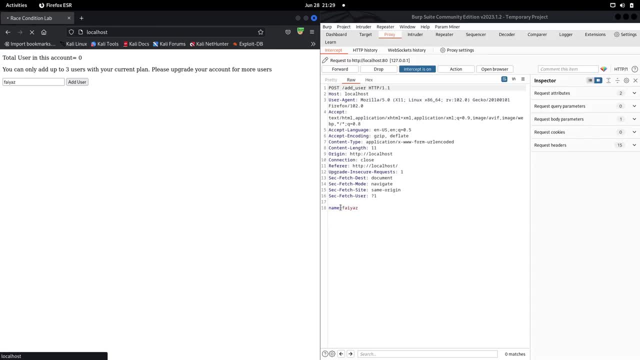 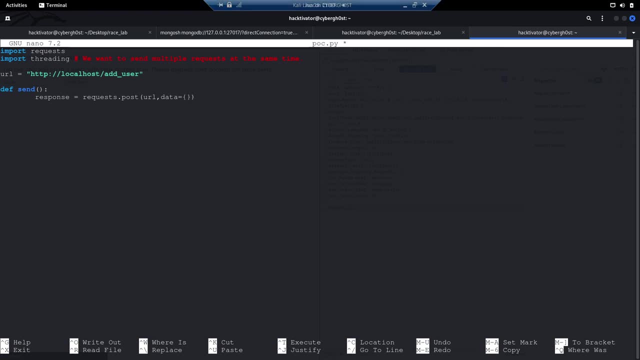 as you can see from here, the parameter is name and then the value. So the key will be name and the value will be the value that we are passing. So let's go with name and let's say attacker. right, then we are going to use the text method. 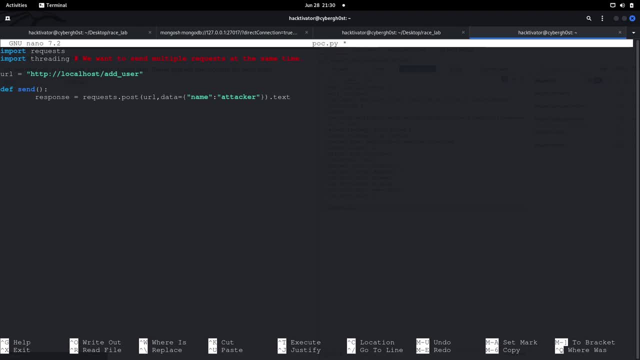 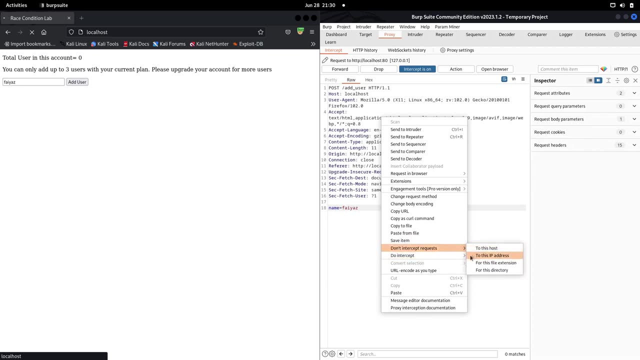 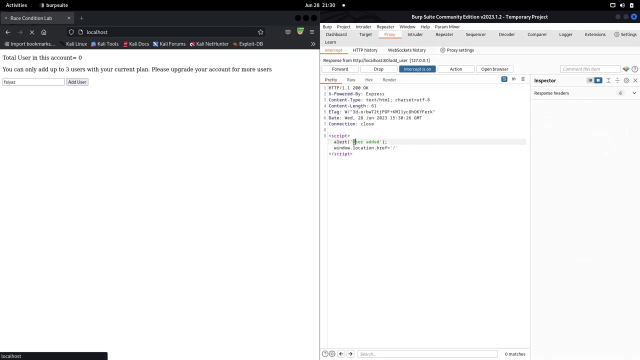 to convert the response into a text format. Okay, we have done that, and now what I'm looking for is: let me just show you So I can just click on. do intercept the response, just forward this and, as you can see in the response, we have a message user added right. So if 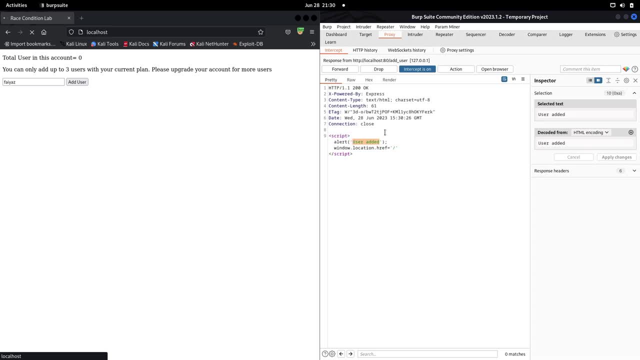 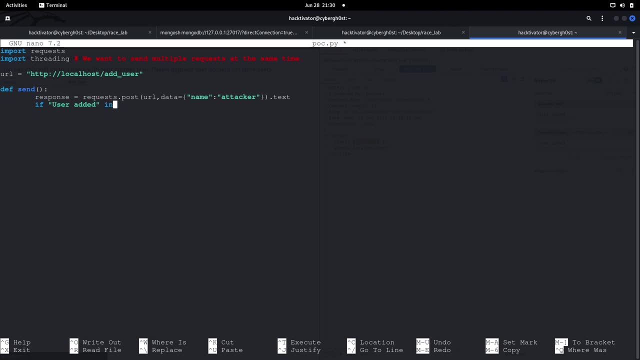 we were successfully able to add a user, then we should be able to see this message: right: user added. So we are going to do: if user added is in the response, then we are going to print: the user has been added successfully, right. otherwise we are going to print. 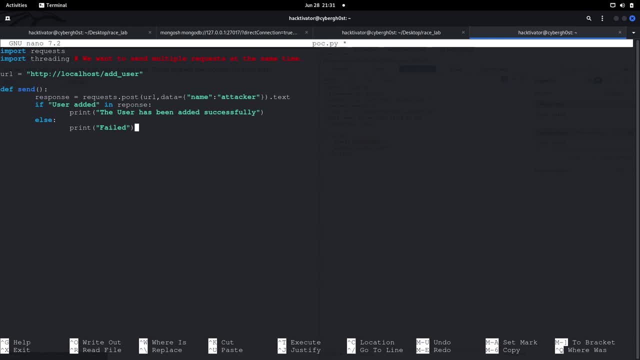 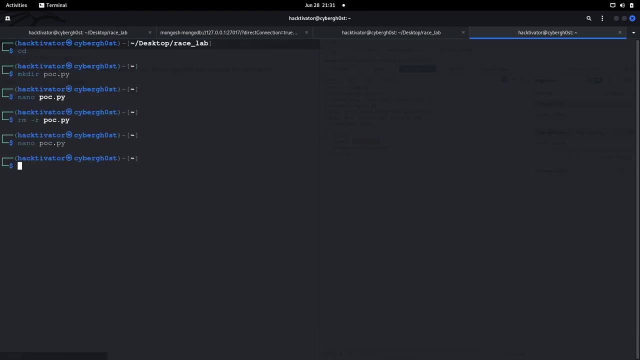 failed. Okay, simple as that. and now let's call this function right. Let's try to run this and if everything works, then we'll be able to see this attacker user in this particular application. Let's run this, pocpy, and we are getting this error. Why we are getting this error? because 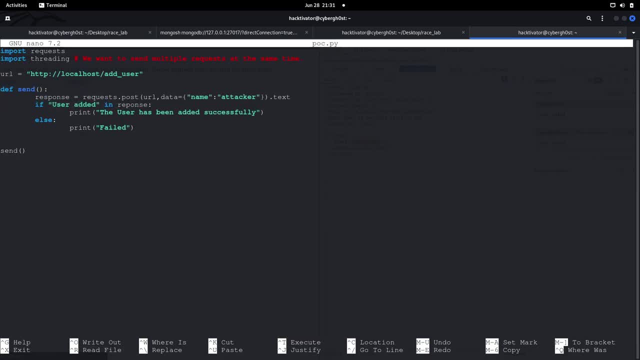 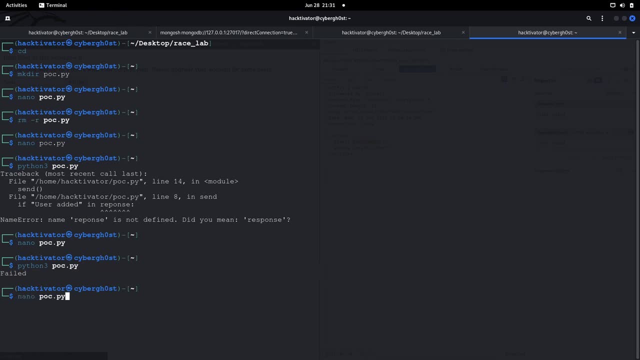 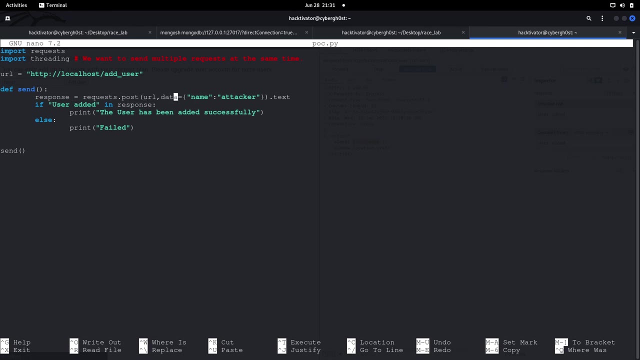 this. there is some spelling mistake over here: res. yes, now we should be able to see it, Showing that it is failed. right, Let's try to see why it is failed. So we have done requestpost, we have sent the URL with the name parameter and all, and. 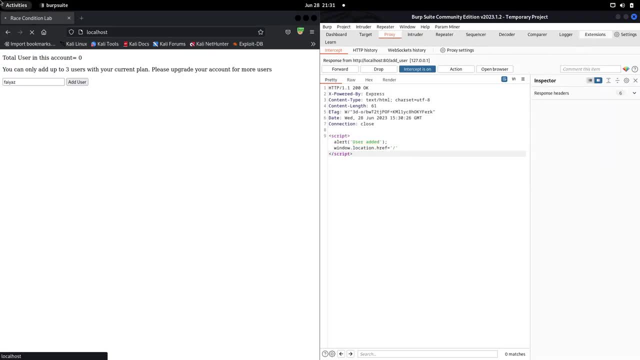 we have think we have done everything right. Yes, So this issue could be. let me just do a quick reset over here. As you can see, the attacker has been added, but we are not getting this. Let me just try to run the python script again. 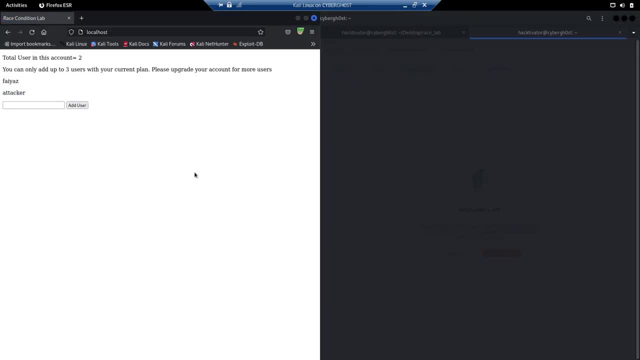 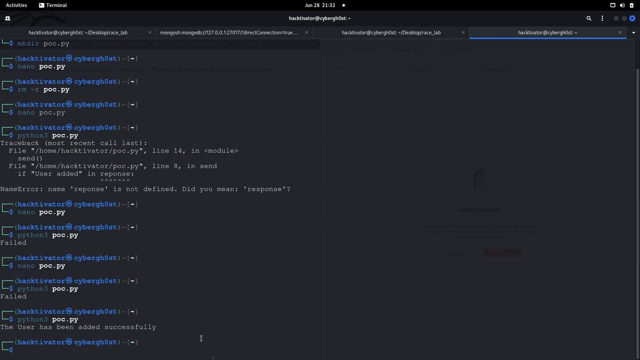 Even though we are getting this error. but yeah, okay, so there is some kind of issue over here. Let me just reset it. Try to run this again. Yeah, showing that the user has been added successfully. Let's test this out. Let's try to run this again. 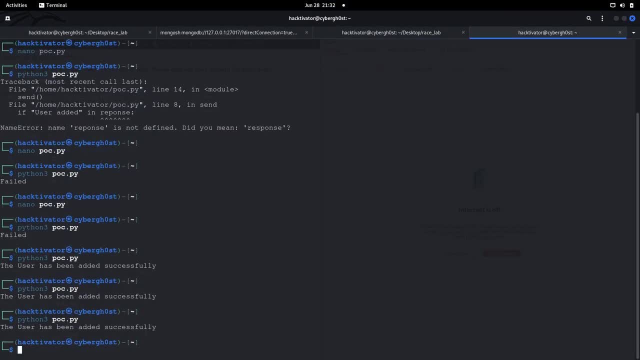 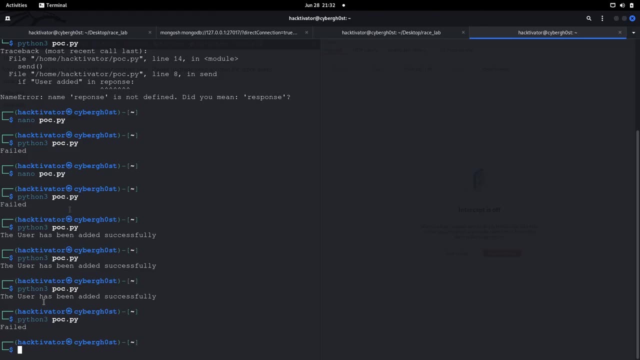 Again, the user has been added successfully, Right? So we should be able to use this tool for three times, right? Because after that it will not allow us to do this. As you can see, now it's showing fail And now we are unable to add any users. 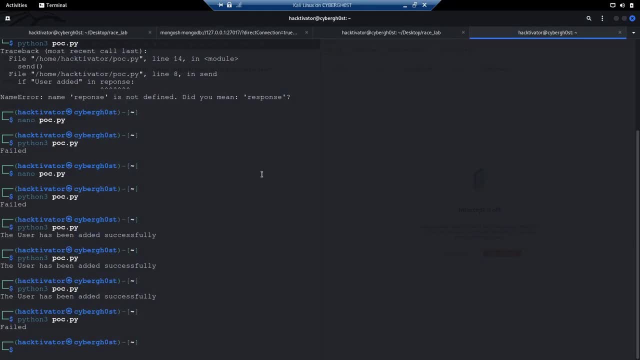 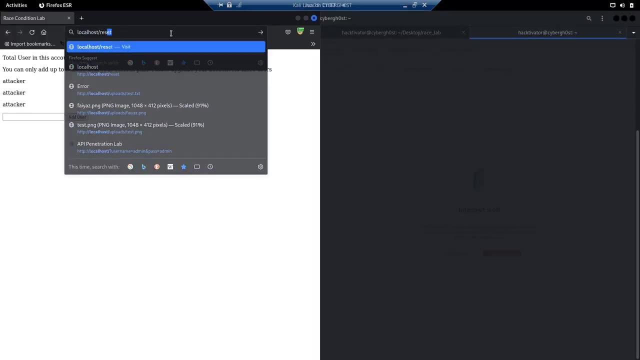 Right, What we are going to do is we are going to speed up this process, The process of sending request. we are going to speed that. Let's see how we can do this, But first let me just reset this back to the initial data. 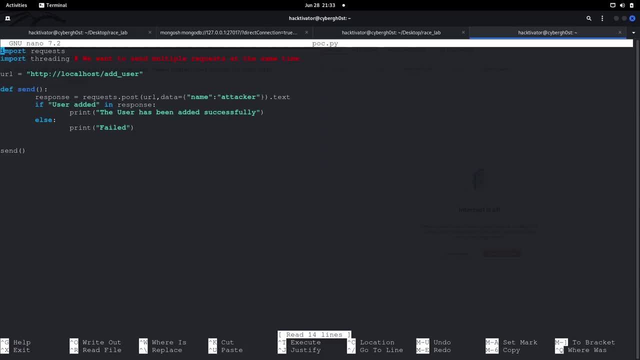 And now we are going to use threading, Right. Let's see how we can do this. So, basically, I am going to create a variable, Let's say a array equals to, And I am going to use a list comprehension method of python. 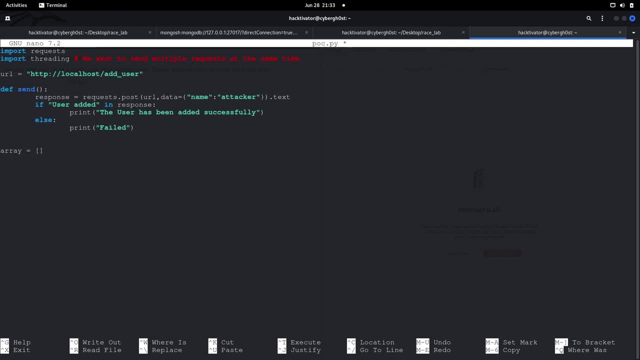 To generate a thousand thread request. that will send this request on the server, Right? So we are going to send thousands of requests at the same time, Right, Let's see how we can do this. So we can type threading dot, thread, dot, target. 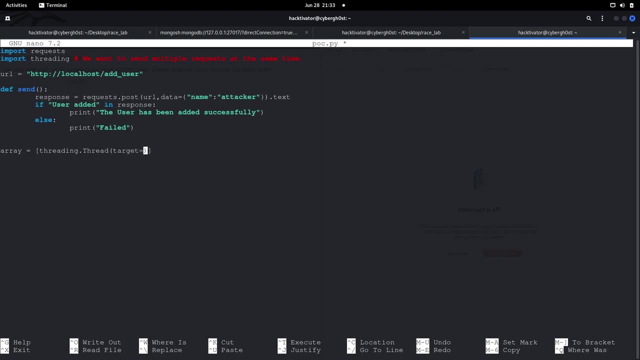 That target equals to this function name, which is send, Right. Then we can just type start to call this function And then we are going to use for x in range thousands, Right? The first thing that it's going to do is it's going to generate a thousands of number. 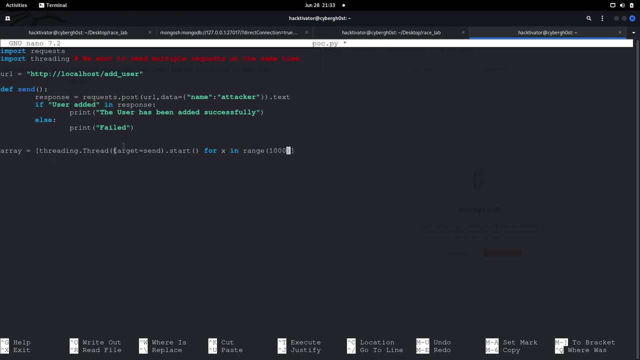 And for each of these numbers it is going to start a thread Right. And what will each thread do? Each thread is going to send the post request on this particular application Right Now. Initially, as you can see that after three attempts we are getting failed. 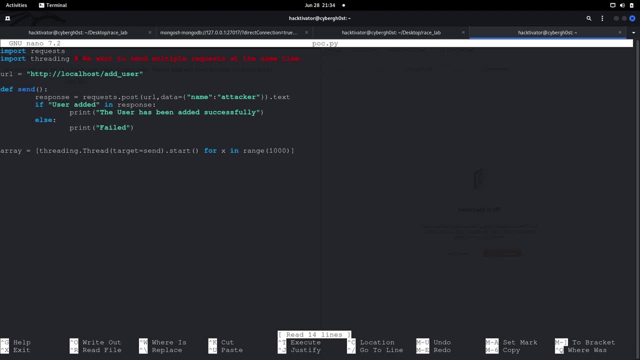 But if we were able to get more of this message- the user has been added successfully- It will mean that we were able to add more users in this application than the actual threshold that has been set Right. Let's save this And let's try to run this. 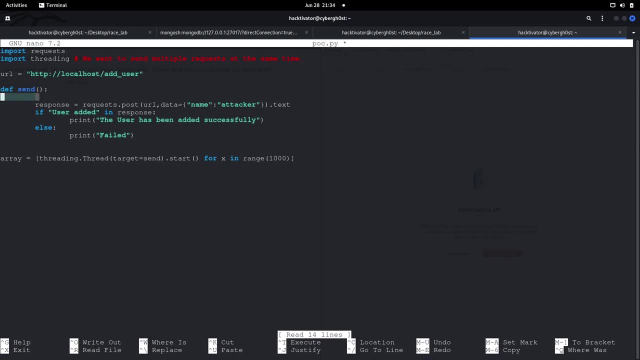 And let's do a small thing as well- That I am going to keep all these things into a loop So that it will keep sending. Each thread is going to send the request again and again, Just to speed up the process, Right? 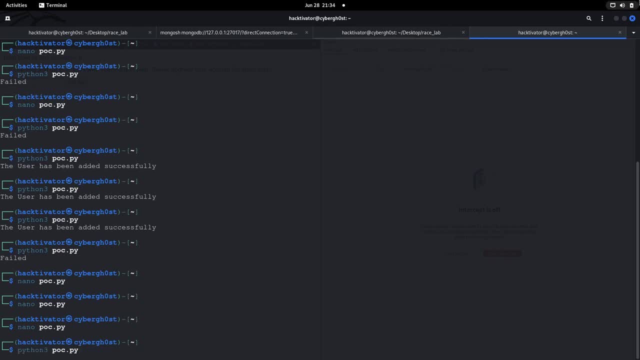 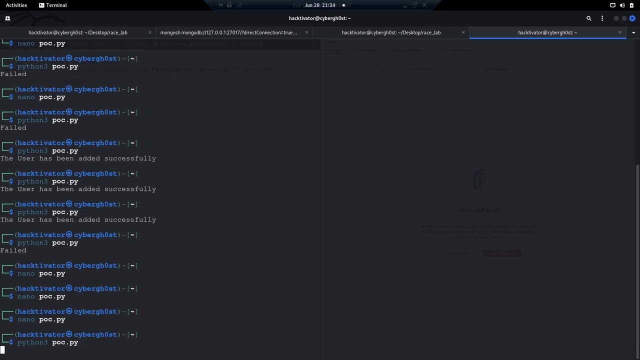 Let's try to run this And let's see what happens. So, as you can see, currently- let me just show you guys that it is currently zero- Let's try to see what will happen if we run this, Run this And now we are getting failed message. Right? 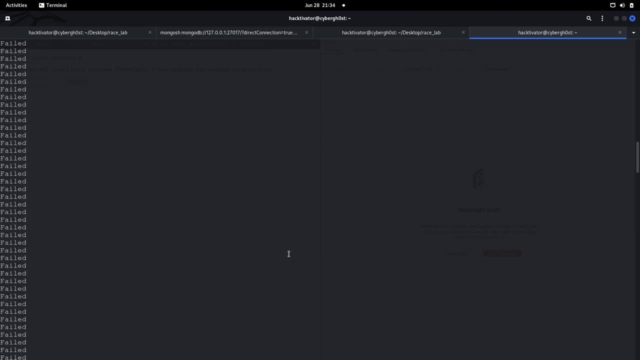 We just stop it right over here And if we look closely up here, We will see that we have got the message how many times: 1, 2, 3, 4, 5, 6, 7.. So we were able to get this message for 7 times. 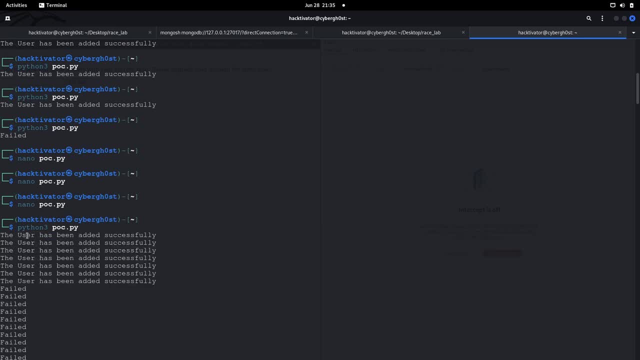 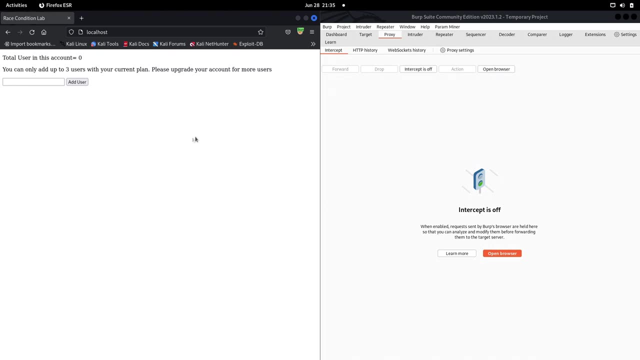 Right. So initially the application allowed us to only add 3 users, Right, But we were able to add how many users? 7 users. Let's try to verify this So we can just refresh this now And, as you can see right over here, 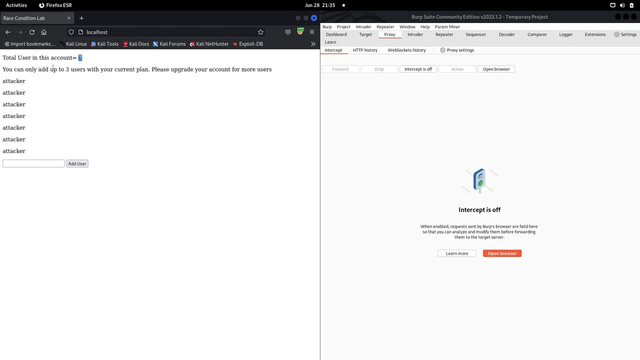 We were able to add 7 users in this particular application, Right? So this is what this condition means, Right? Why this is happening. Let's try to understand this in the source code. Let me just open the source code And we are going to see how we. 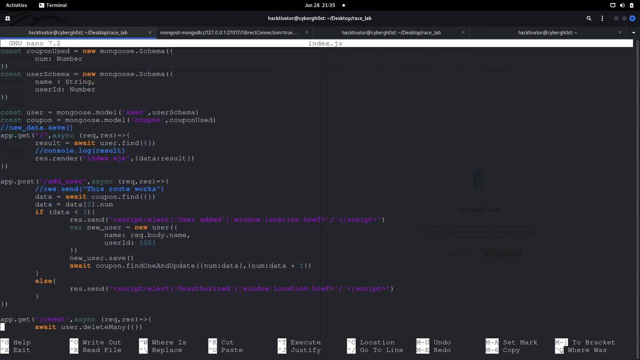 What is the actual cause behind it, Right? So see, This is the post request going on, Right? First thing that it is doing is It is finding the amount count. basically, Right, Suppose that if I have added the user one time, then the count will increment to 1.. 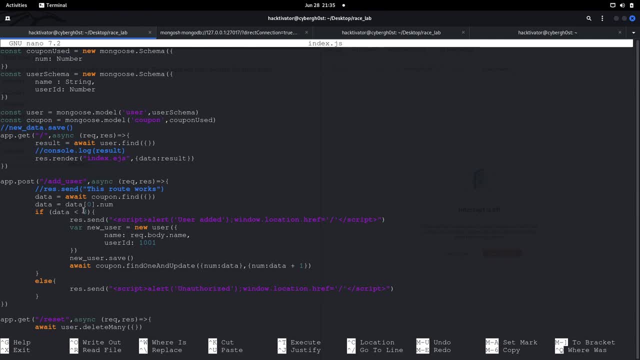 Then it is checking the count, whether the count is less than 3 or not. If it is less than 3.. Then it is adding this, Right, And then it is incrementing the data, Right. So suppose I have added a new user. 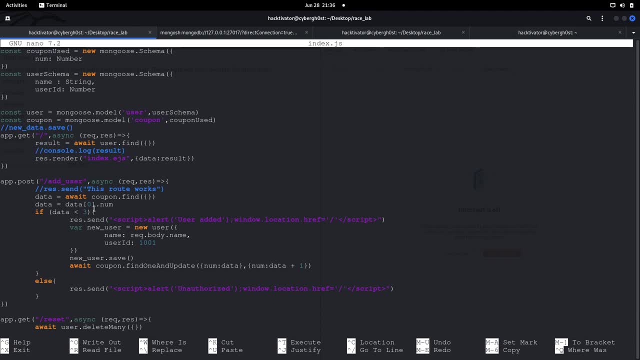 Then the value will be incremented to 1.. So the initial- Let's say the initial- user I have is 0.. I have added a new user, So the new user will become 0 plus 1 equals to 1. Right. 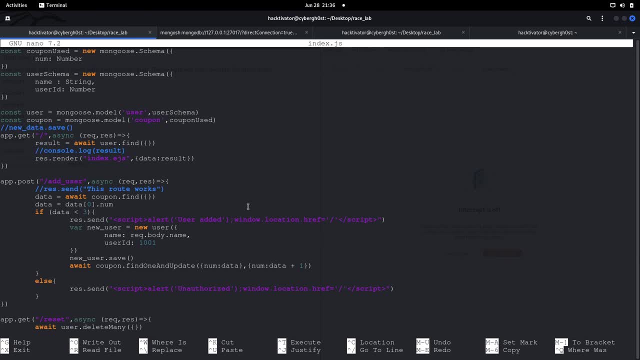 The new count will become 1. Right. Similarly, if we add new user, Then it will become 1 plus 1 equals to 2. Right. Otherwise, If the data is greater than 3 or equals to 3. Then we will get that we are under authorized to access this server. 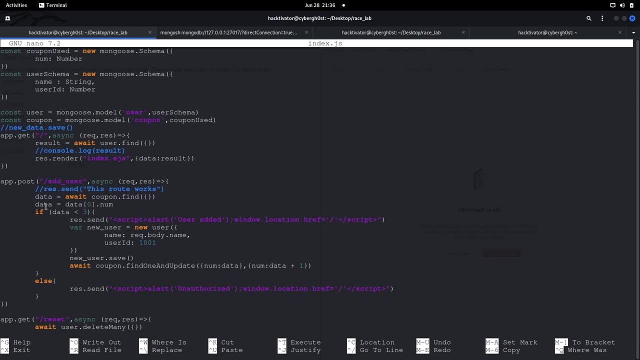 But the thing over here is: See, Between this time, Between this, first it is going to check the data, Then it is going to say user alert, Then it is going to add the data And then it is going to increment the data. 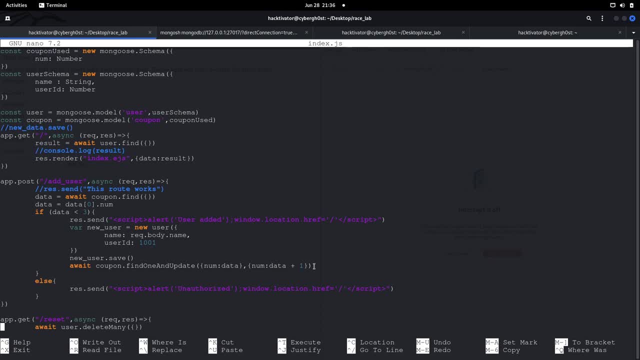 Right, But if multiple threads are working, Then it could be possible that, Let's say, two or more threads were able to read this data When the data's value is 2. Right, So now, Instead of one thread, Two threads have read the data. 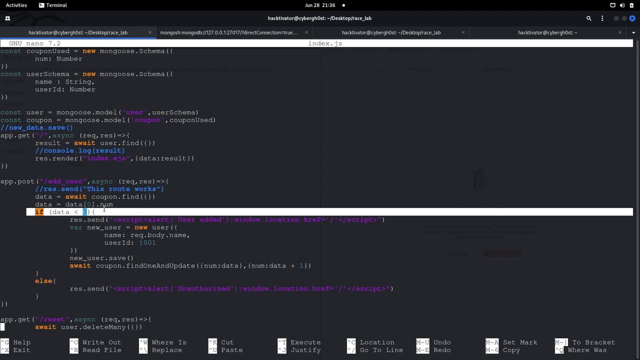 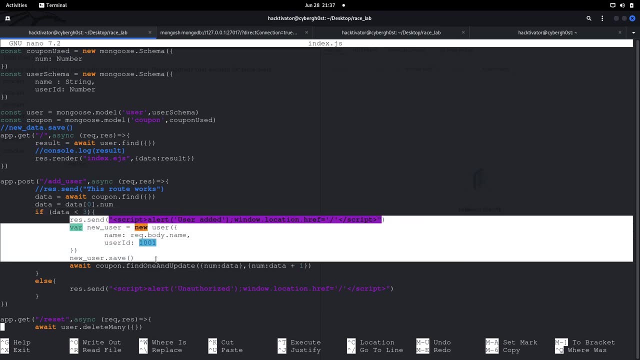 That data is 2. Which is less than 3.. Right, The two threads were able To read this data, Which means That the two threads will be able to create users, Which means that There will be two users created. 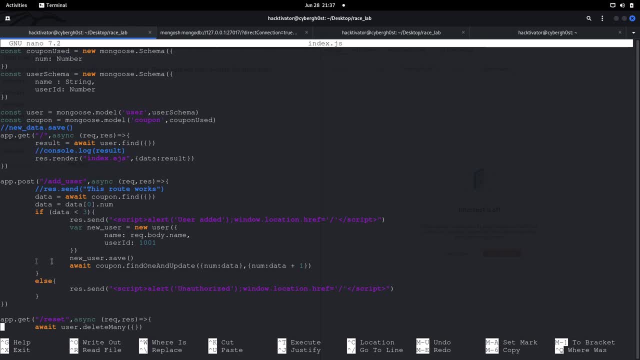 For the value 2.. Right, I hope you were able to get along with me. Basically, There is a time delay Between verifying and uploading the file, So if multiple requests were sent at the same time, Then We will be able to. 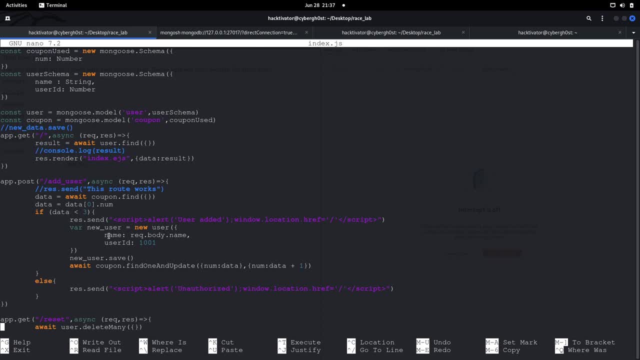 Do some stuffs Like the logical vulnerability that we did over here, Right? So this is the actual cause of this application And if you have Saw- Also on my previous video, In which I have shown you that How we can bypass the file upload restriction- 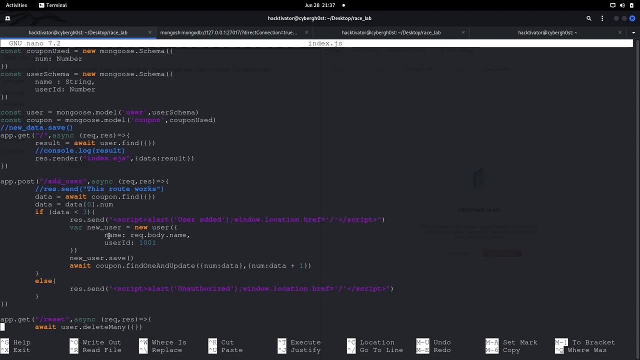 Using the same race condition method. Then you know how it works, Right? So if you haven't checked this, Check that video out. Then the link is given in the description. You can also check that one out, Or also you can see it on the right side of the screen. 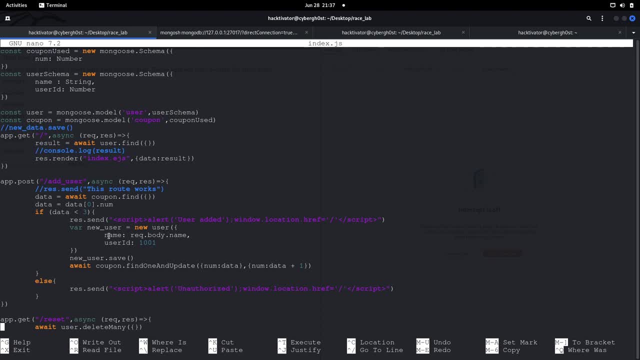 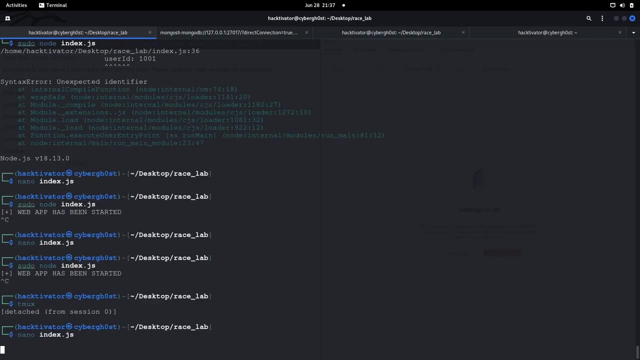 Right? So this is the main reason behind This particular vulnerability, Which is race condition, Right? I hope that You have understood it. Feel free to let me know If you have any doubts Or any issues, Right? So this is basically. 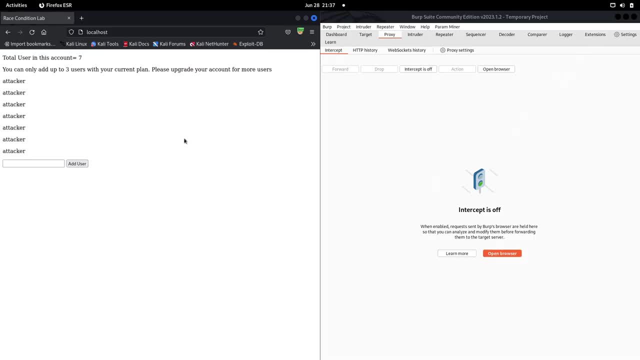 How you can look for Race condition vulnerability Now. the question Is: How do you Look for Race condition vulnerability Now? the second question Is: Where should we look for Race condition vulnerability? Right, As you can see from here. 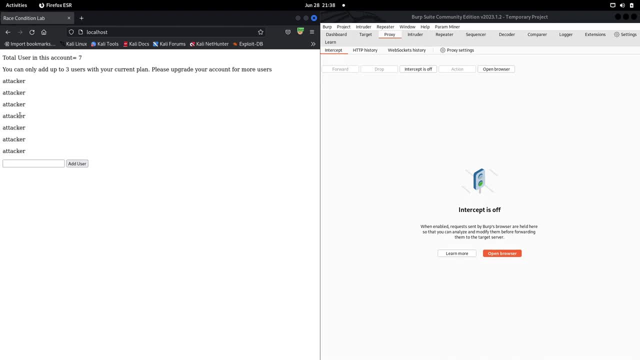 Look for vulnerabilities: Race condition vulnerabilities, Basically, Where The application has some limits. Like You can add up to 3 users, You can use this coupon only once. You can transfer 1000 amount of rupees At only.